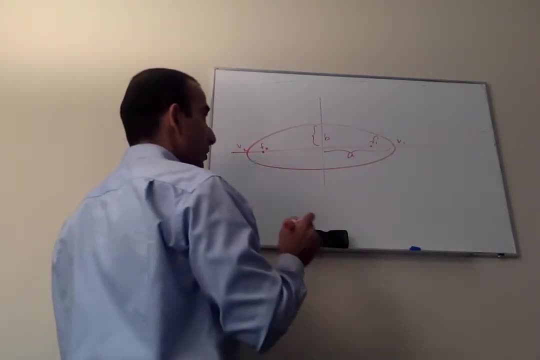 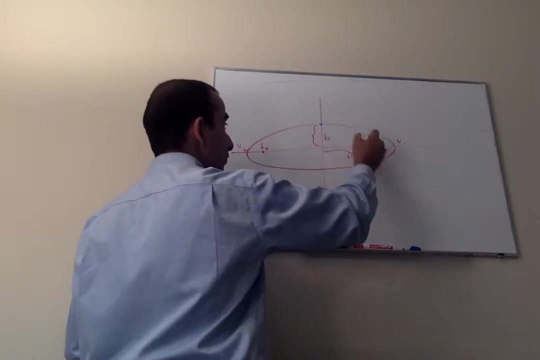 very often. but that's a confusing statement, So I'm going to break that down a little bit by using a particular point. So if you take this point, the distance from foci 1 to this point we could perhaps call D1.. And the distance 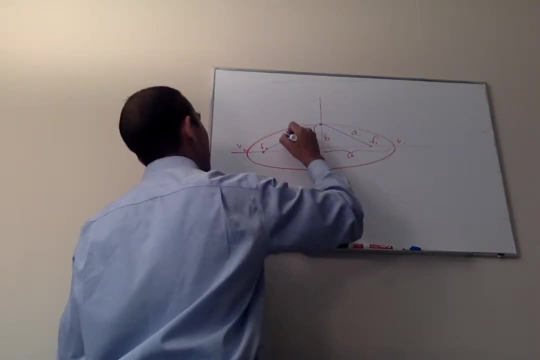 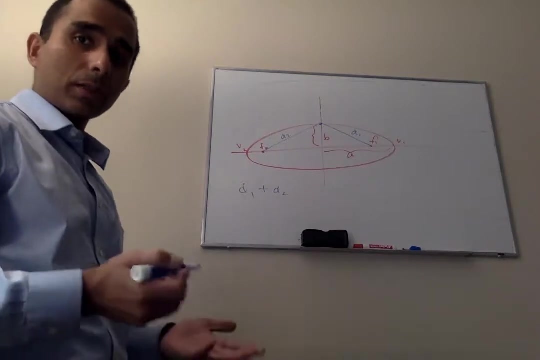 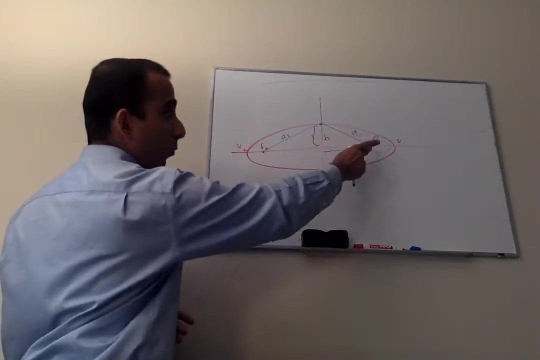 from foci 2 to this point we could call D2.. By definition, D1 plus D2 is constant. That's the definition of an ellipse. An ellipse is the collection of all points where D1 plus D2 is the same, Where D1 is the distance from foci 1 to the point and D2 is the distance 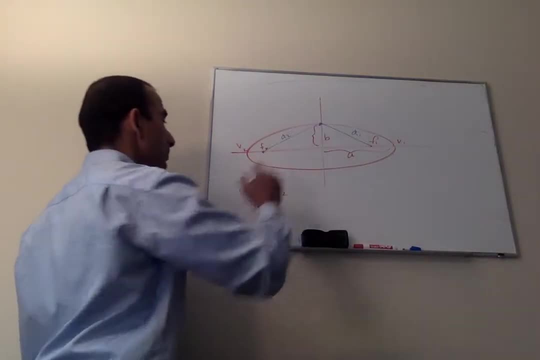 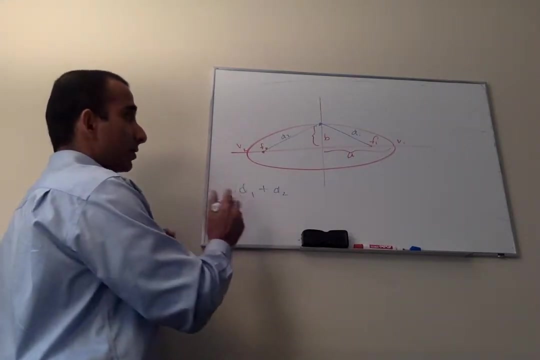 from foci 2 to that same point. So if D1 plus D2 is constant, we should be able to get the same distance from the foci at any point in the ellipse. So let's for instance now take vertex 2.. The distance: 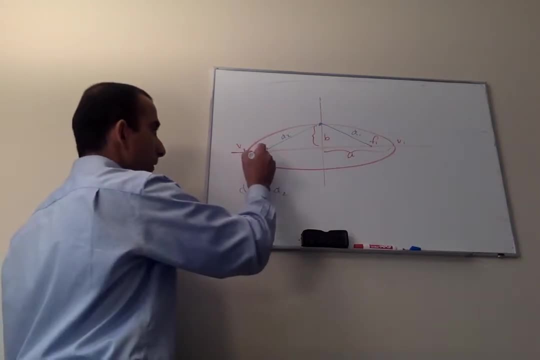 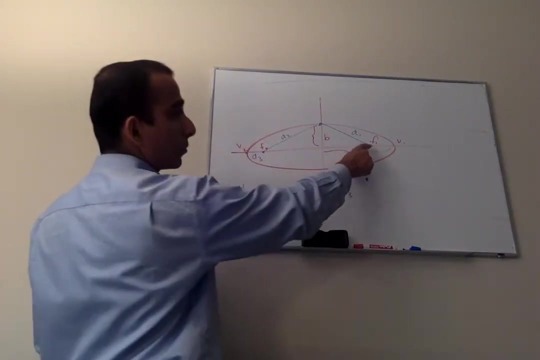 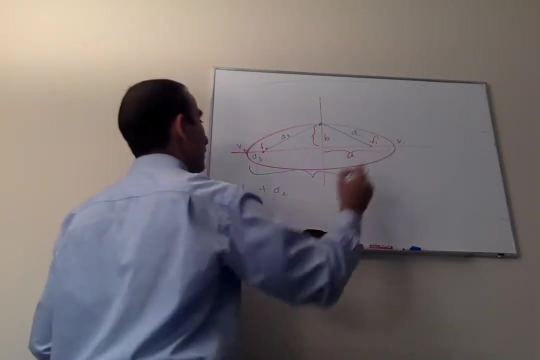 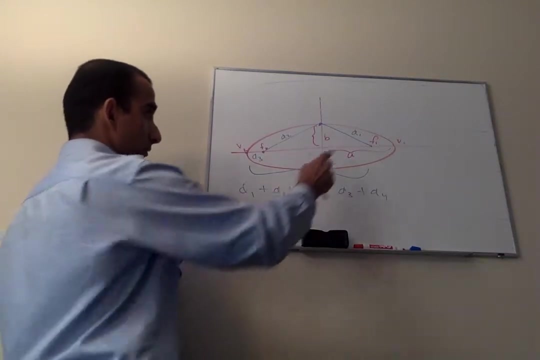 from focus 2 to vertex 2, let's call that D3.. Um, and the distance from focus 1 to vertex 2, I'll mark it over here in blue: this distance over here, let's call that d4.. So, from what we just said, d3 plus d4. 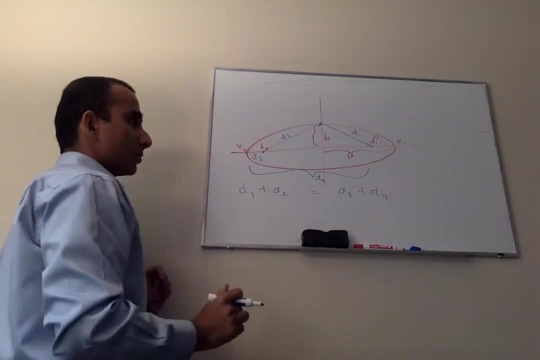 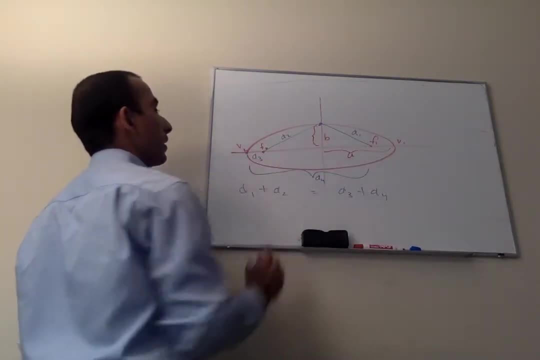 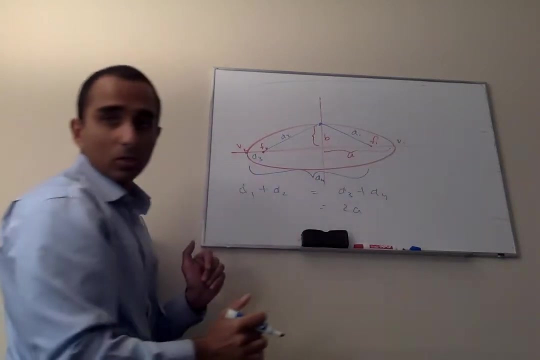 have to equal d1 plus d2.. But you can see over here that d3 plus d4 is also equal to 2a, because this is a and this is a, and d3 plus d4 is the entire horizontal axis, That's. 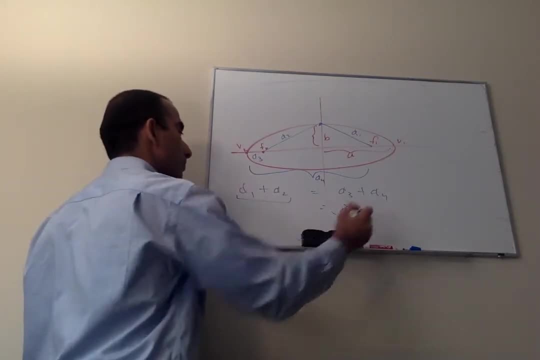 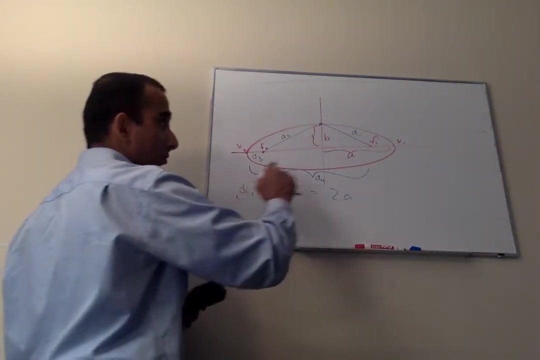 the proof, the basic proof, of why d1 plus d2 is equal to 2a. right Now let's look at that one more time. So b1 plus d2 is equal to 2a a plus a. But we know that d1 and d2. 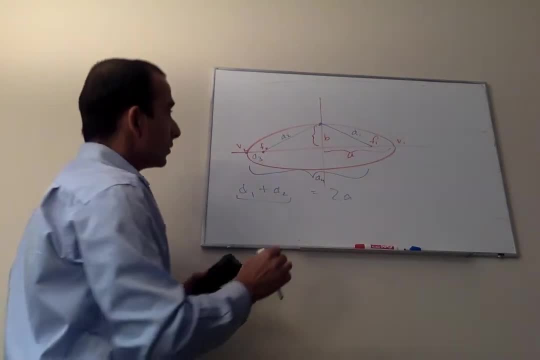 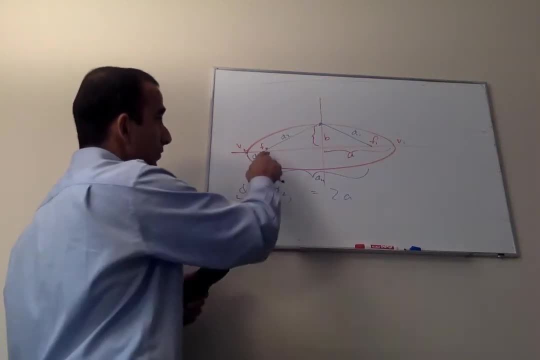 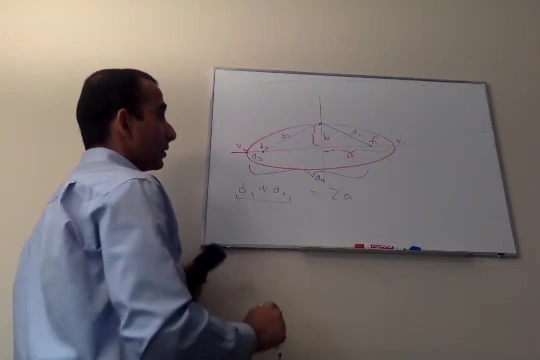 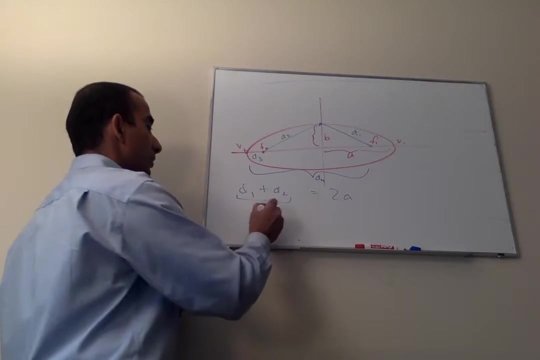 d2 are equal. So we know that d1 and d2 are equal. So we know that d1 and d2 are equal In this particular case because the foci is symmetric about the central axis, d1 is equal to d2.. So if d1 is equal to d2 and d1 plus d2 is equal to 2a, then we know that. 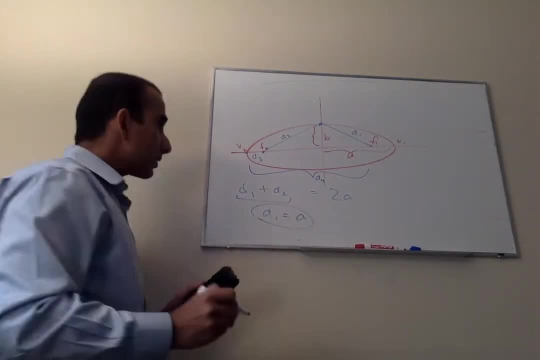 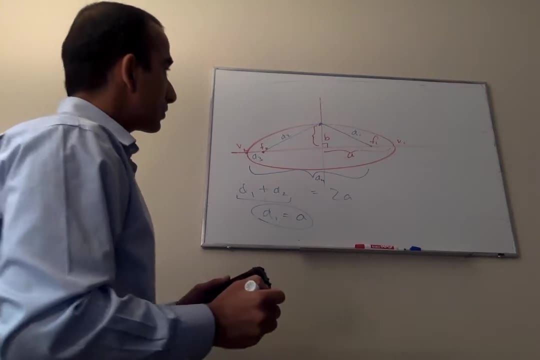 d1 is equal to a, And that's the key to solving our equation for the focal distance. So now that's it. I know now that d1 plus d2 is equal to total. d1 plus d2 is equal to 2a. 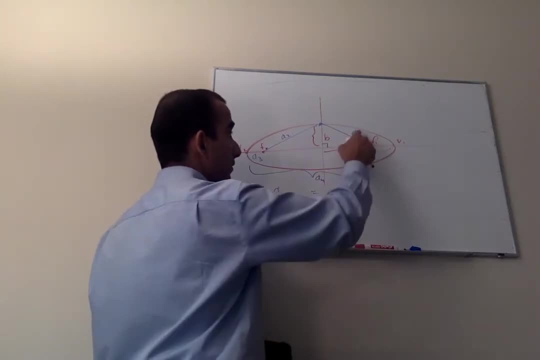 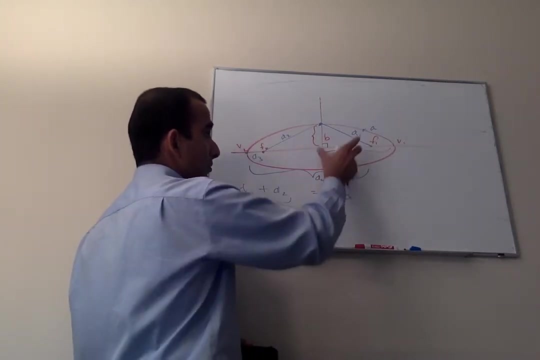 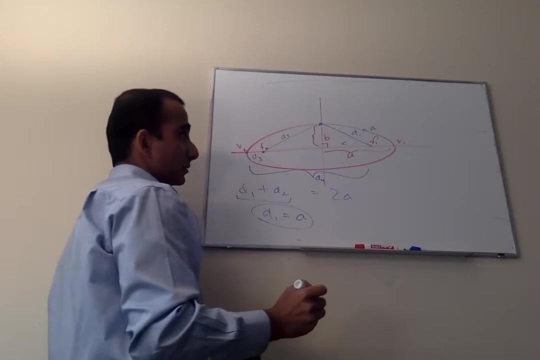 So now we can write this항 Stuff. we can rewrite a and d1 is also a, So I can just replace this. I can just write an a over there, d1 is a. Now, this distance over here we can call c, this distance right here, That's the distance from the center of the ellipse. 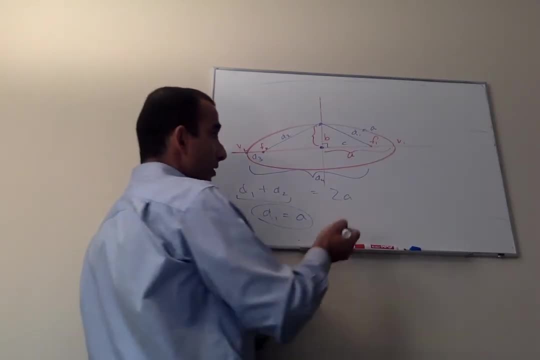 to the focus. It's also called the focal distance. So from this you know from the Pythagorean theorem that d2 is equal to 0. And c is indeed aouls. So this distance down is d2, d2 is. 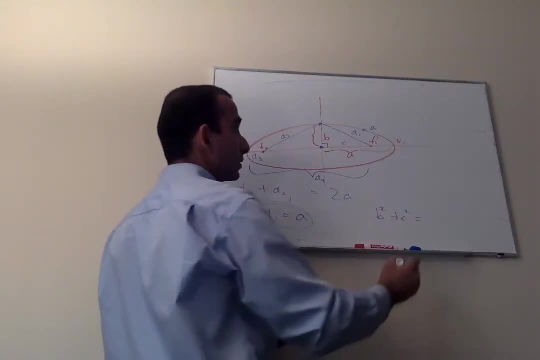 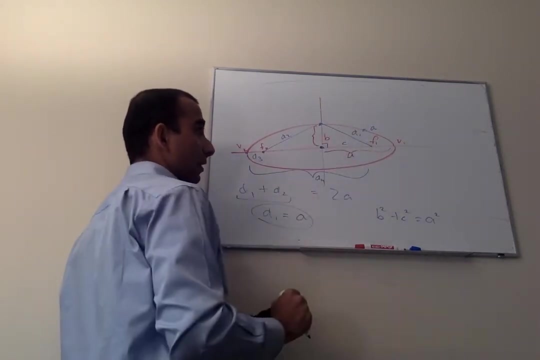 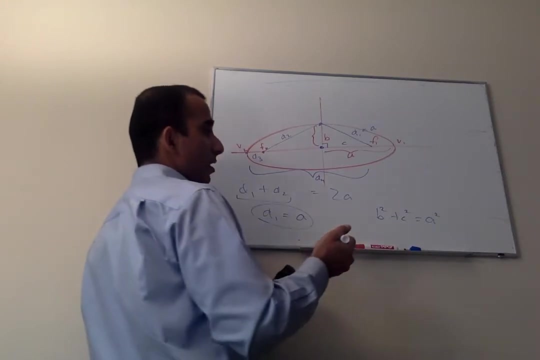 b squared plus c squared is equal to a squared or d1 squared. That's the Pythagorean theorem: b squared plus c squared equals a squared, because a is also d1.. This can also be written as very often, the way it's written as c squared is equal to a squared. 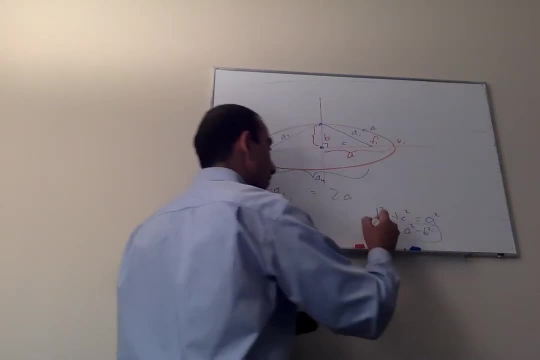 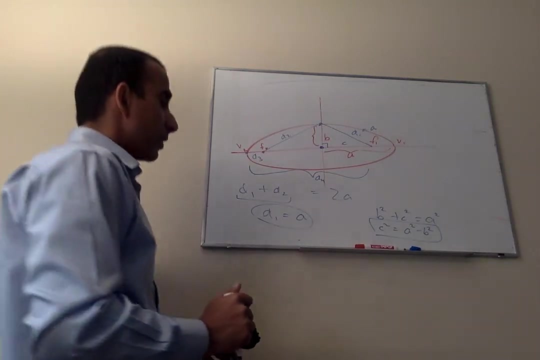 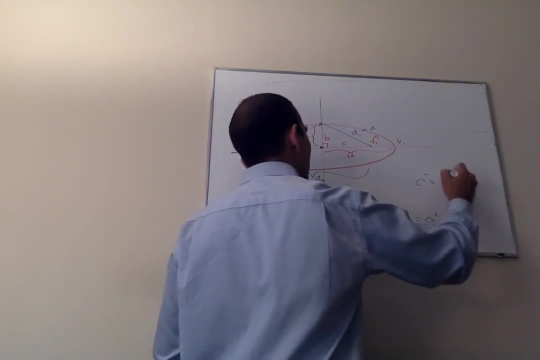 minus b squared, And that's the way to find the focal distance in an ellipse: c squared equals a squared minus b squared. If you have an ellipse that's vertically aligned, then that equation becomes: c squared equals b squared minus a squared. Okay, so that's ellipses. We're going to do hyperbole next.